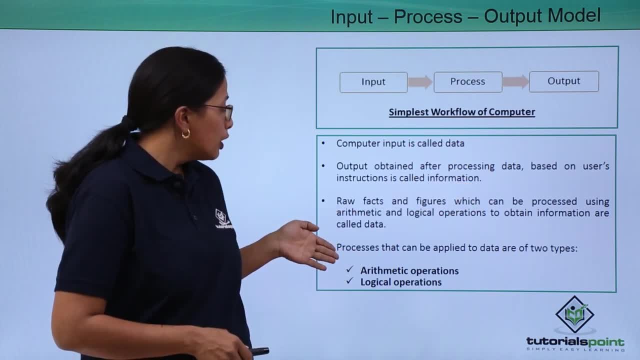 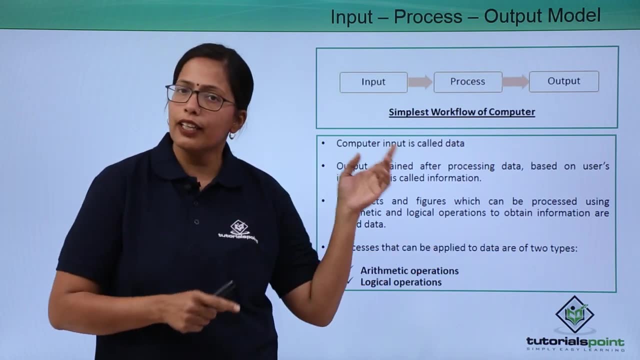 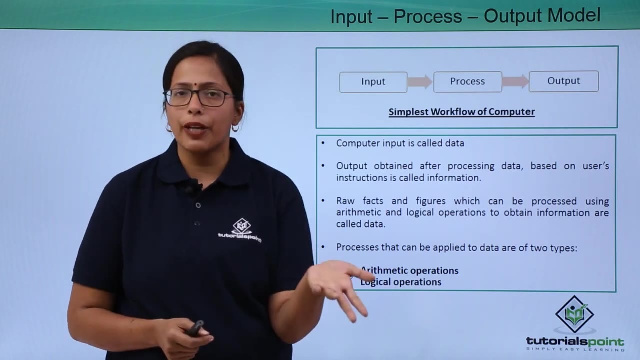 the computer. So this brings us to the processes that can be applied to. the data are of two types: Arithmetic and logical Arithmetic. an example I have given you just now: addition, subtraction, multiplication. What are logical operations? If I want to compare something, I give two numbers and 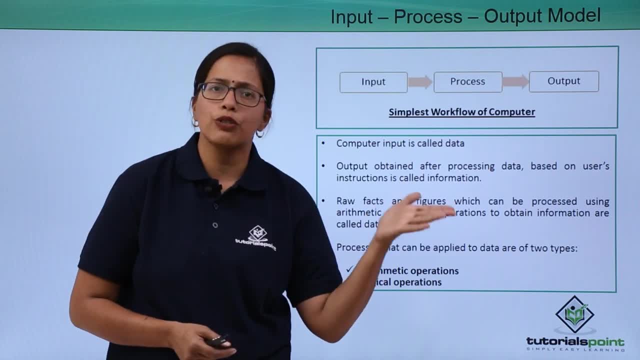 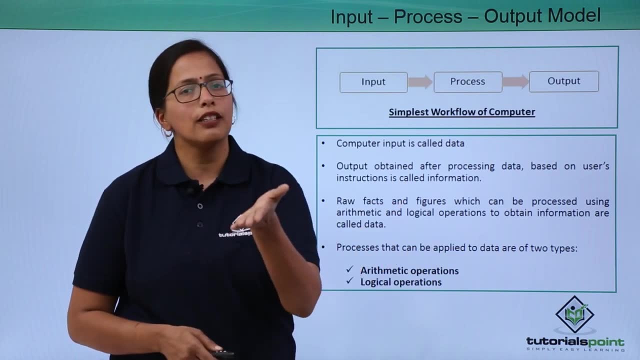 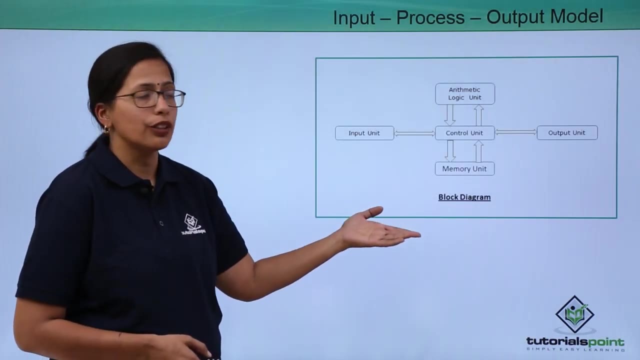 I ask the computer to say which is greater. So I give the same two numbers, 2 and 3. but my instruction is: compare to two numbers and tell me which is greater. So it will tell me the answer as 3.. So that will be a logical operation. This is the actual model of the computer, the block. 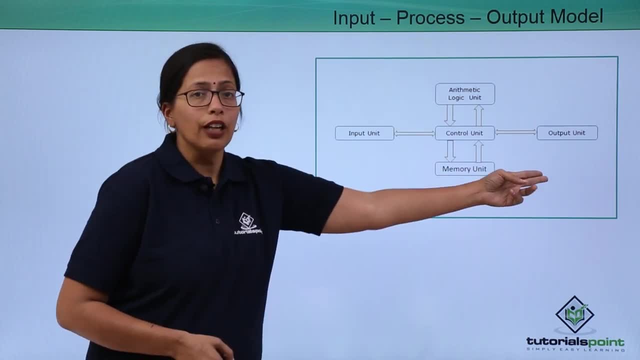 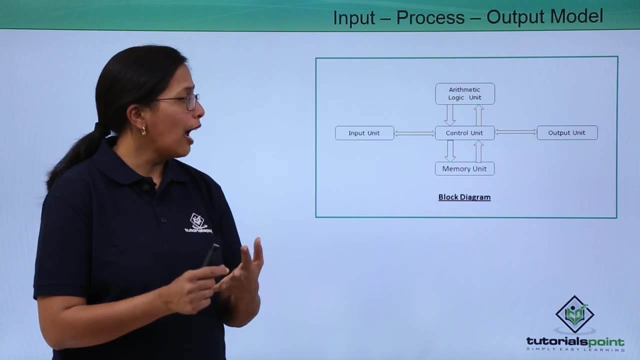 and the output. So this is the formula, the basic part of the computer, and out is overall the input unit. We have an input unit here and we have an output unit here. However, the processing unit has three separate units: the arithmetic logic unit, the control unit and the memory unit. 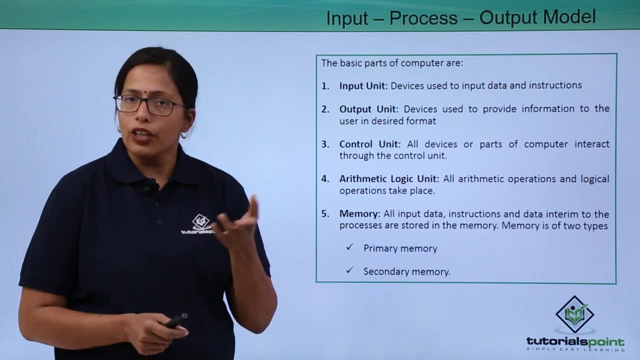 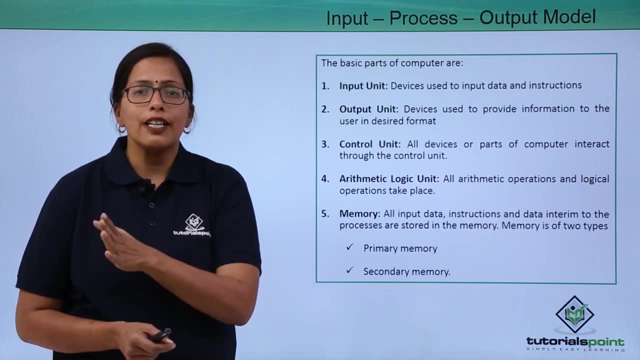 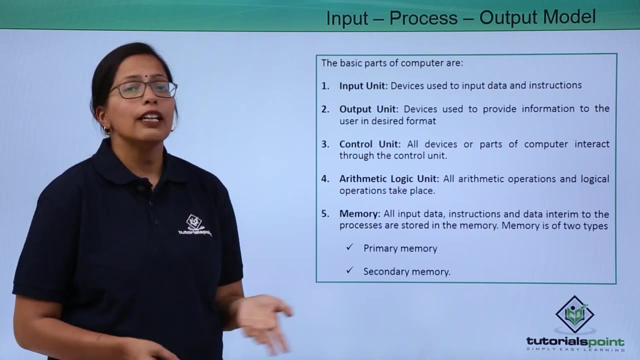 Let's see how all these basic parts of computer are functioning. The input unit: it consist of the devices that are used to give data or instructions to the computer. The control unit: the control unit is of all the parts of the computer. The arithmetic logic unit: it carries out all the arithmetic operations and logical 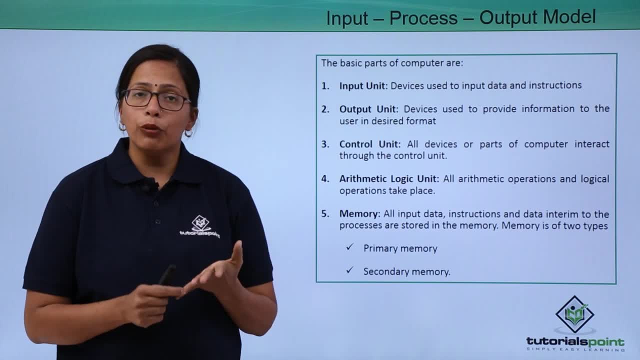 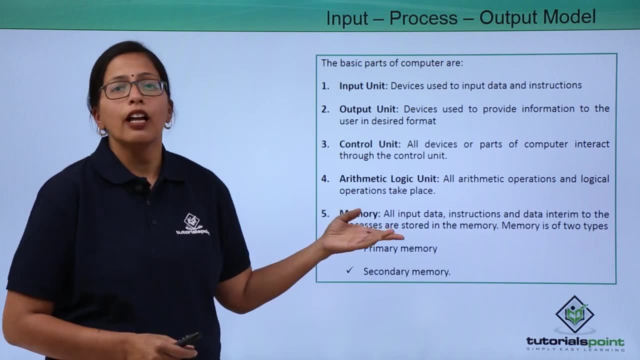 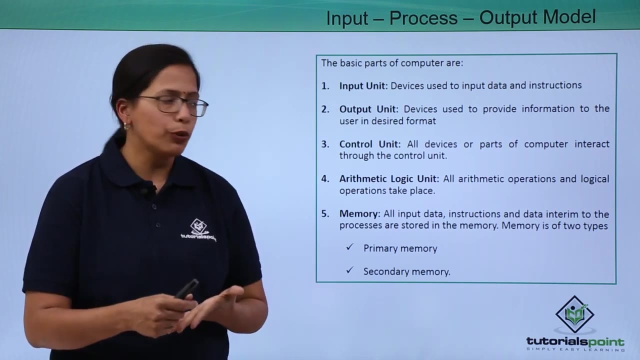 comparisons: The memory, all the input data, instructions, output. the interim data is stored in the memory unit and, finally, the output unit. The devices that are used to give us output are the output unit. The memory is of two types: primary memory and secondary memory. 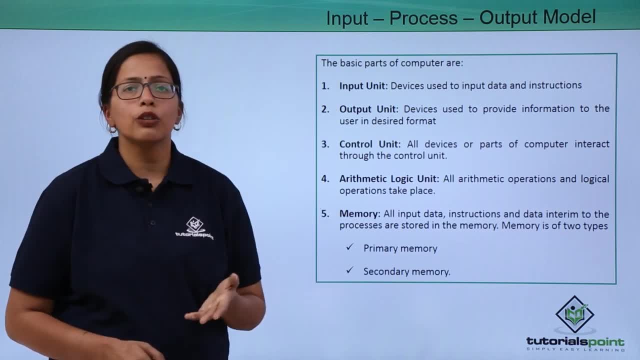 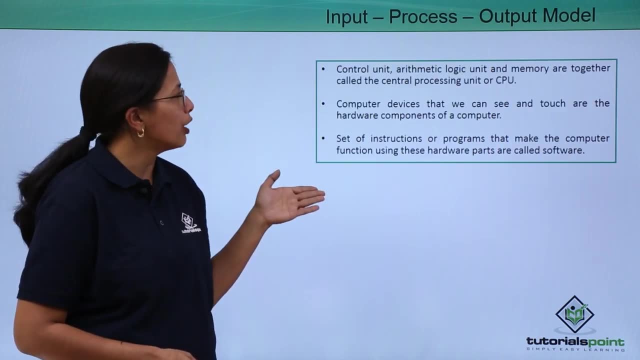 Input unit could be your keyboard or mouse. the output unit could be your printer or your monitor. These are some of the things that you should keep in mind about a computer. The control unit, the arithmetic logic unit and the memory unit are together called the. 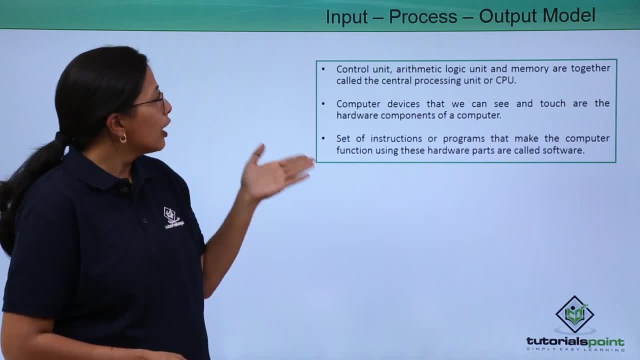 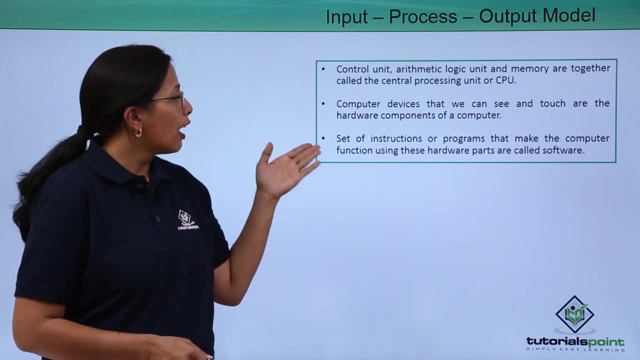 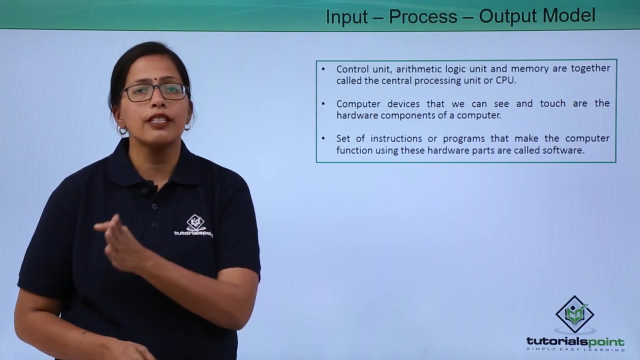 CPU or the central processing unit. Computer devices that we can touch and feel like a keyboard, a mouse. a keyboard, a computer monitor, a mouse are called the hardware components of the computer. Besides the hardware component, a computer also has software.